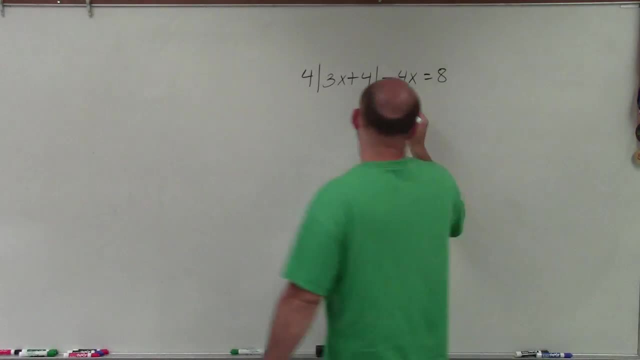 my absolute values being multiplied by 4 as well as being subtracted by 4x. So I'm going to undo each of those. So I'll add 4x to both sides first. Then I have 4. absolute value of 3x plus 4 is equal to 4x plus 8.. Then I undo the multiplication of 4, so I divide. 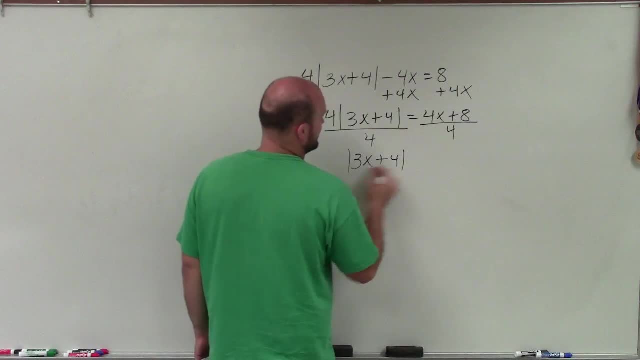 by 4.. And I have 3x plus 4. absolute value is equal to 4x divided by 4, which is going to be x- sorry, 8 divided by 4, which is positive 2x. And now you can see I have my absolute value isolated. So therefore, again I need to create: 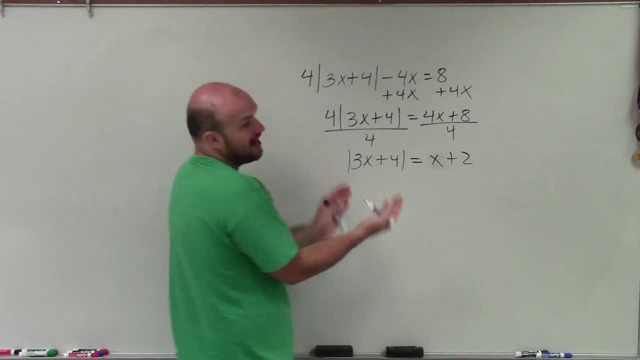 my two cases, one where the value inside my absolute value is positive and one where that value is negative. And to do that, when we create our two cases, we can now kind of get rid of the absolute value, because that's exactly what the absolute value is telling us is this: 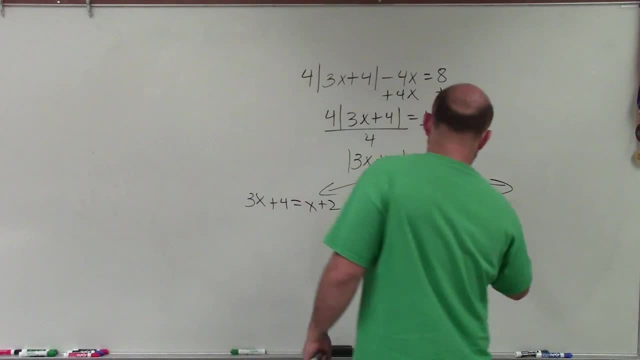 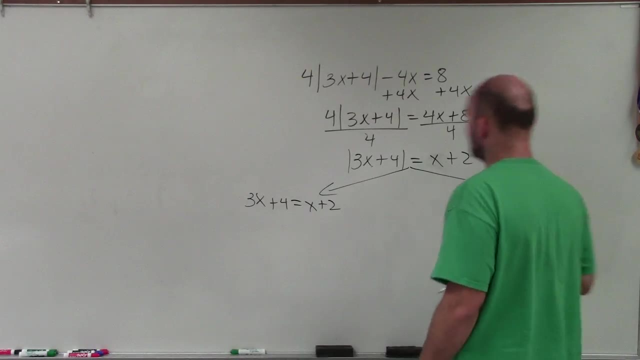 value could be positive or negative, but it's going to have the same solution. So that's the case for the positive. To write the case for the negative, what I'm simply going to do is just take the opposite of my other side. 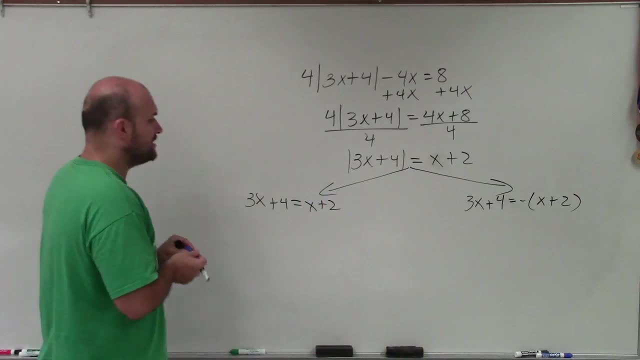 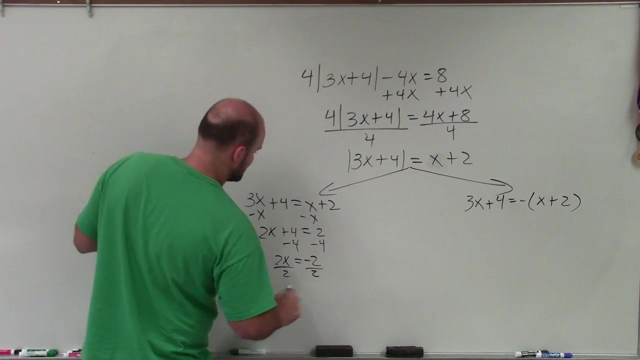 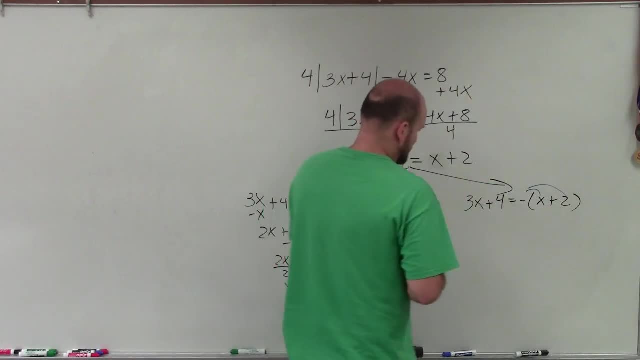 make sure I distribute my negative sign. So I have here: 3x plus 4 is equal to a negative x minus 2.. Then again, solve for my x's. So I add an x onto both sides, So I have 4x plus. 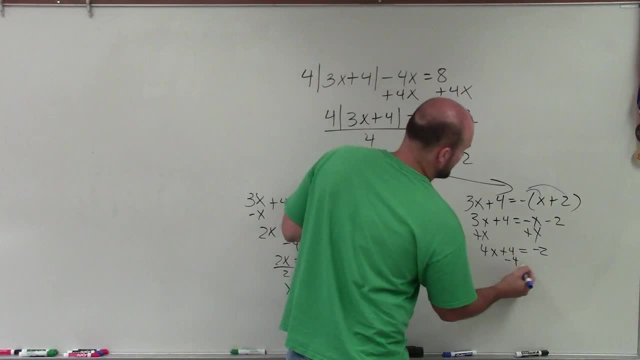 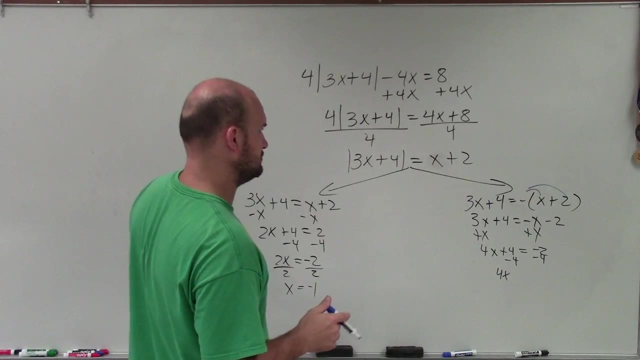 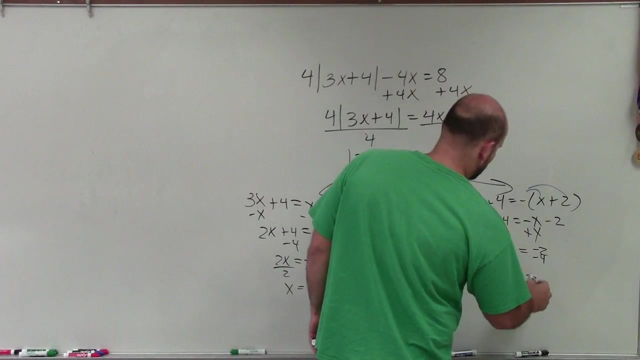 4 is equal to a negative 2. Again, subtract 4, subtract 4, 4x. Added an x. add an x, 4x. Okay, 4x is equal to- I did this- negative 6, divide by 4,. divide by 4, x equals that's. 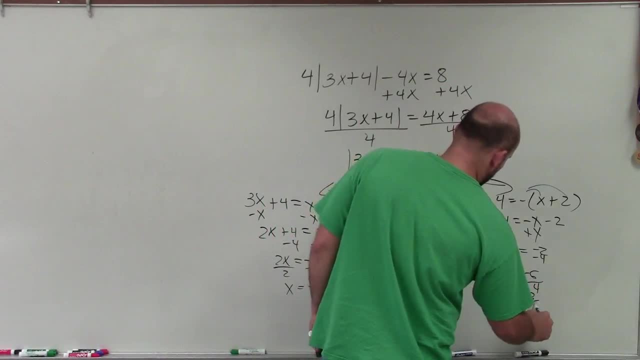 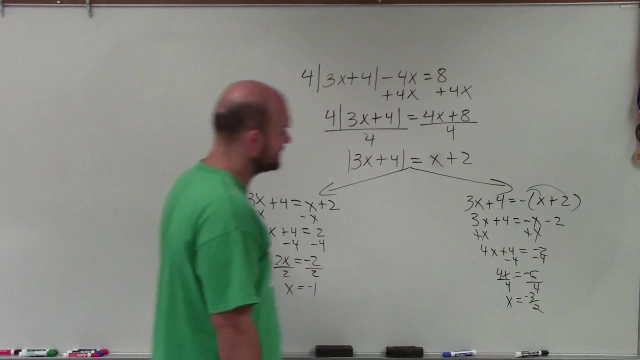 a positive 6,, isn't it? No, it's a negative 6. Equals a negative 3: halves, Alright. well, I guess we'll see where it goes. So again, let's go ahead and plug in now to test each. 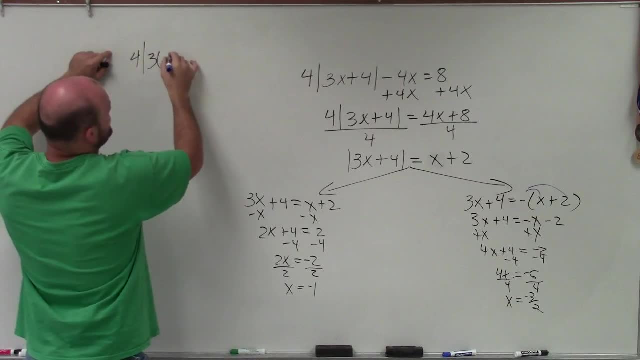 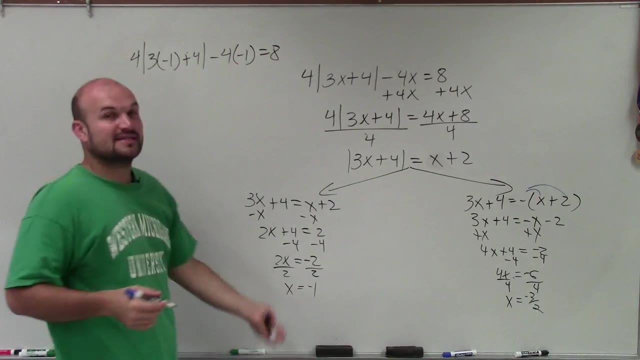 one of these solutions. I have 4 times 3 times negative, 1 plus 4, absolute value. minus 4 times negative, 1 equals 8, right, So you're going to take your value and plug it back into your equation and see if it works Well, 3 times negative, 1 is negative 3 plus. 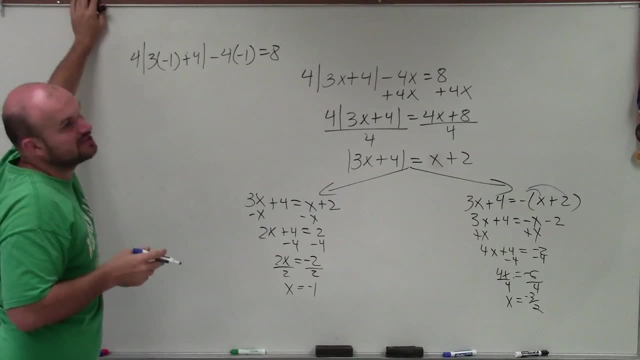 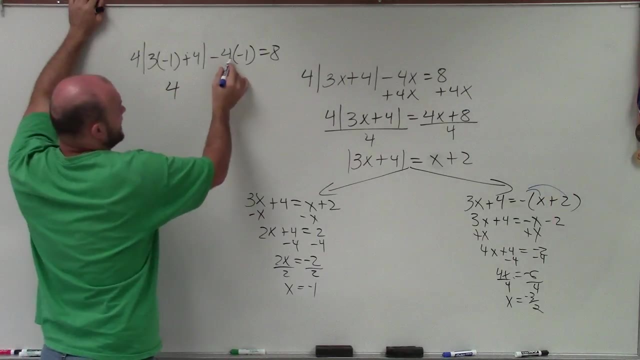 4 is going to be negative. 3 plus 4 would be positive: 1. Absolute value of positive 1 is still 1, right, And then times 4 is going to give you 4.. Negative 4 times negative 1. 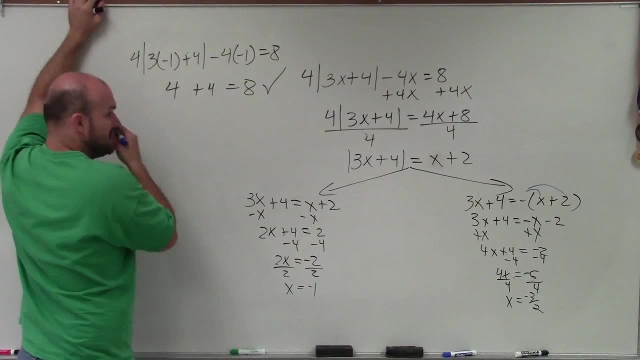 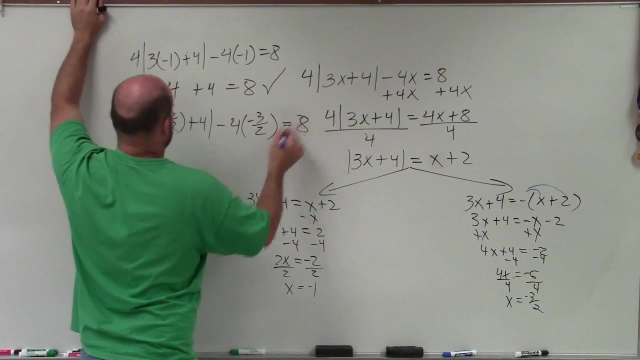 is a positive 4, equals 8, and you can see, yes, that works For the second case. now I need to plug in a negative 3 halves. So I have 4 times 3 times negative 3 halves plus 4, minus 4 times negative 3 halves equals 8.. Alright, 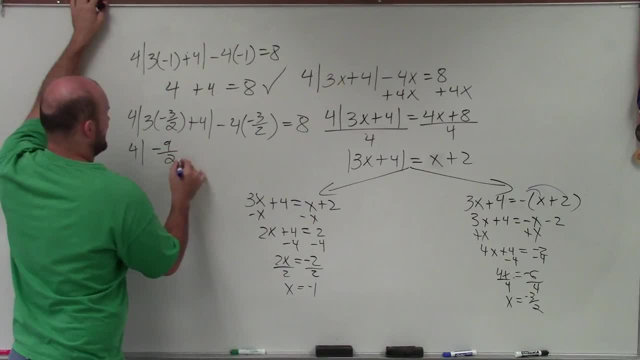 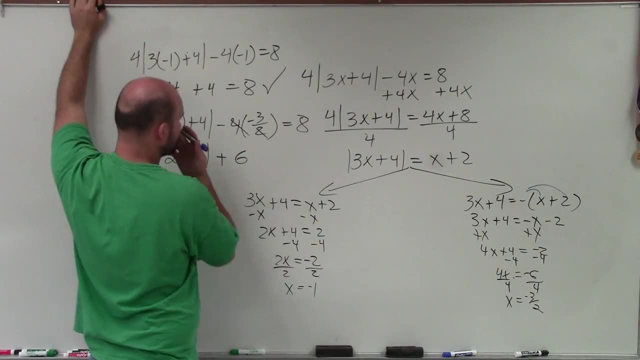 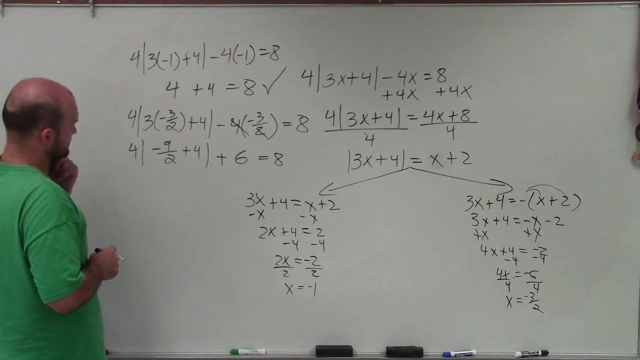 so I have 4, absolute value. this becomes a negative. 9 halves plus 4, minus. this becomes a positive 6, equals 8.. This is really 8 over 2, right 4,, when written as a denominator, is 8 over 2, so it's 4, absolute. 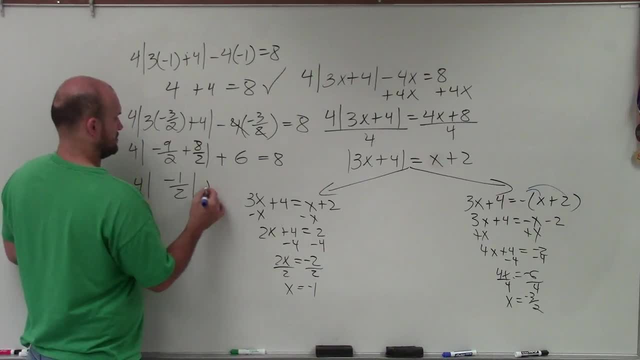 value of negative 1 half plus 6, equals 8.. Well, negative 1 halves is the value of a negative, 1 half is positive, 1 half Positive, 1 half times 4 is just going to leave you with a 2 plus 6 equals 8.. And guess what, ladies and gentlemen, With even checking it, 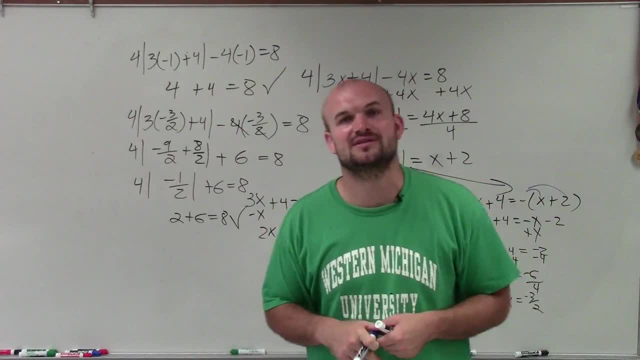 out with fractions, we still go ahead and verify that both of those are going to be your solutions. Thanks,